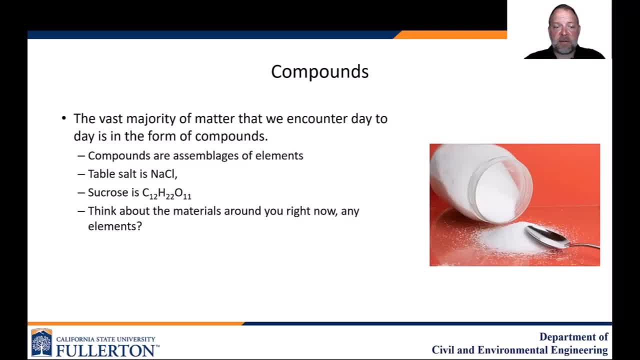 The vast majority of matter that we encounter day to day is in the form of compounds. Compounds are assemblages of elements. We talked before about how elements are the very basic, fundamental building blocks of matter, and compounds are when those elements are assembled together. One compound that you're familiar with is table salt, that's sodium. 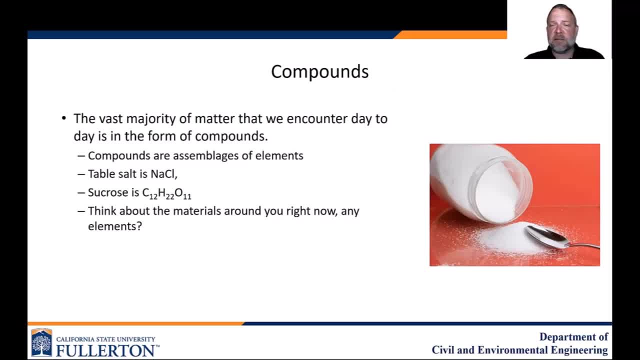 chloride, NaCl Sucrose. another compound that you're commonly familiar with, table sugar is C12H22O11, so it tells us that the way that carbon hydrogen and oxygen bond in sucrose is a 12 to 22 to 11 ratio. Now think about the materials around you right now. Do you think you are being exposed to? 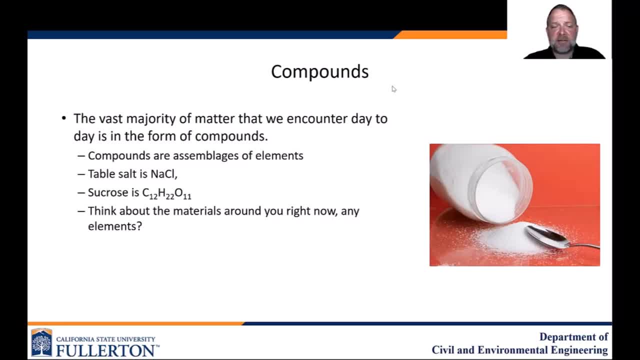 any elements. As I said before, the vast majority of matter that we encounter is in the form of compounds. You can only think of one element that you might have been in contact with technically- two, but one you might not know about. You can only think of one element that you might have been in contact with technically- two but one you might not know about. 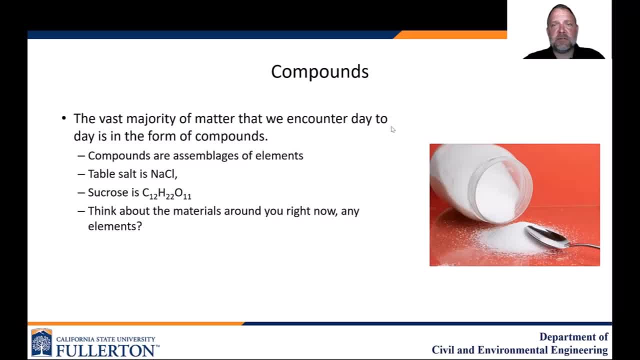 You can only think of one element that you might have been in contact with technically two, but one you might not know about, And that would be gold. If you have 24 karat gold jewelry, that is just gold, It's not bonded with. 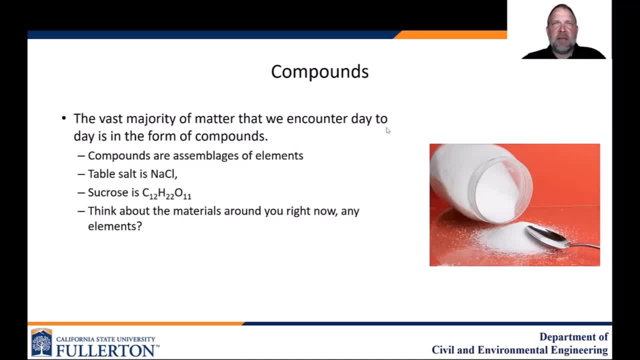 anything else, it's gold held together with metallic bonds, But silver, you know, most silver is actually only 95%, so there's other things in there too, so that would make it a compound, Even the air that you're breathing. So, like I said, aside from jewelry, I don't think you're. 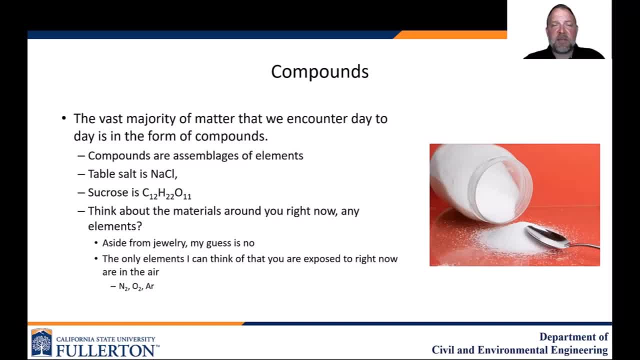 really encountering any elements right now, except the only one that you are encountering is argon- that I can think of at least. So even nitrogen, So the air that you're breathing nitrogen is N2, it's actually a compound of two. 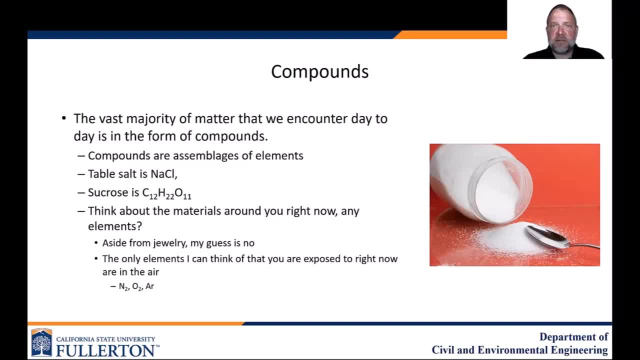 nitrogen atoms. Oxygen is a compound of two oxygen atoms: it's O2.. Argon is a noble gas, and it's roughly one percent of the atmosphere that you're breathing right now. So, yes, you are being exposed to one element all the time, but that's probably about the only one, at least at a 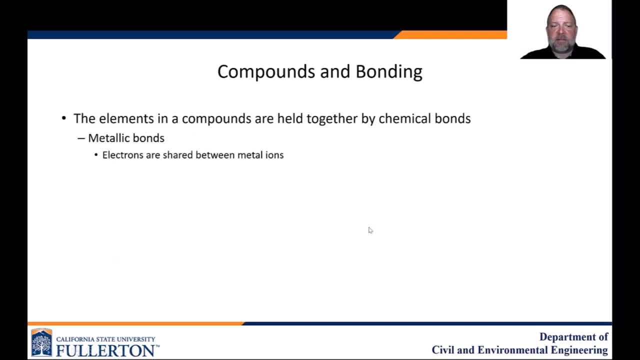 level that you can observe or notice. The elements in compounds are held together by chemical bonds. One is metallic bonds, that's when you have electrons shared between metal ions. One is covalent bonds: electron pairs are shared between atoms when the outer shell is either full or nearly empty. 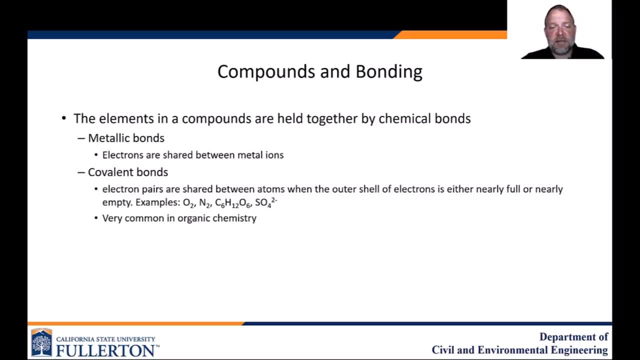 either nearly full or nearly empty. Examples are oxygen nitrogen, that's C6H12,- sorry, that's glucose- blood sugar and sulfate SO4, 2-. It's very common in organic chemistry. that's why I use glucose as an example. 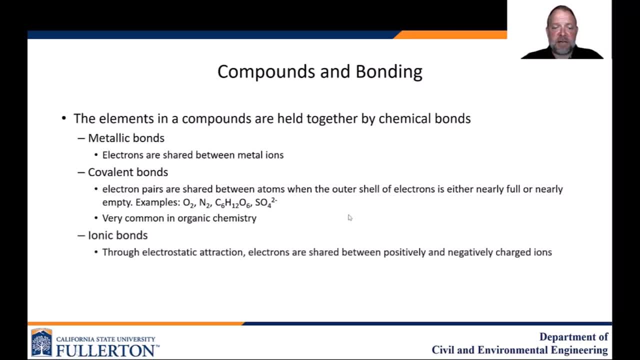 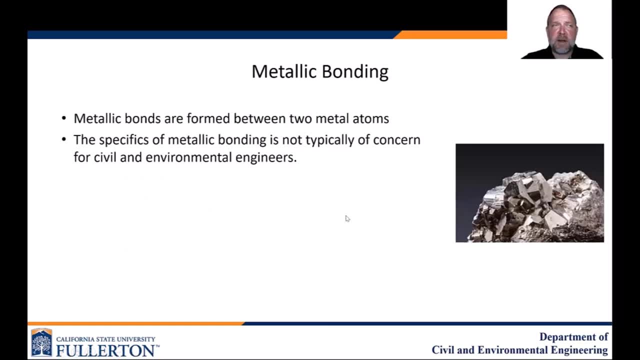 Ionic bonds are actually bonds through electrostatic attraction that are shared between positively and negatively charged ions. That's really common in inorganic chemistry. So organic chemistry is often covalently bonded, inorganic chemistry generally ionically bonded. So, as I said before, metallic bonds are formed between two metal atoms. The specifics are: 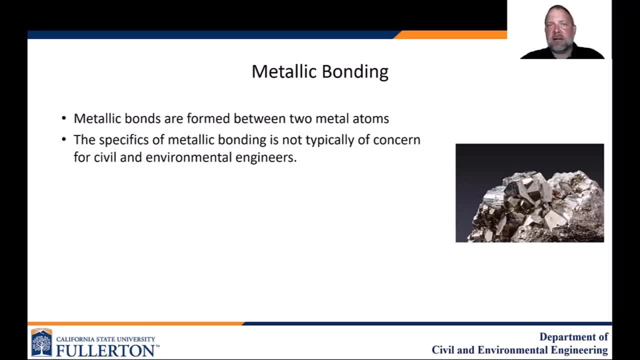 actually not really of concern for civil and environmental engineers. We don't really care how the metallic bonds are being formed. What we do care about is the bulk material properties. We want to know how dense it is, how strong it is, how stiff it is. So Young's modulus is a stiffness For what it's worth. those are those. 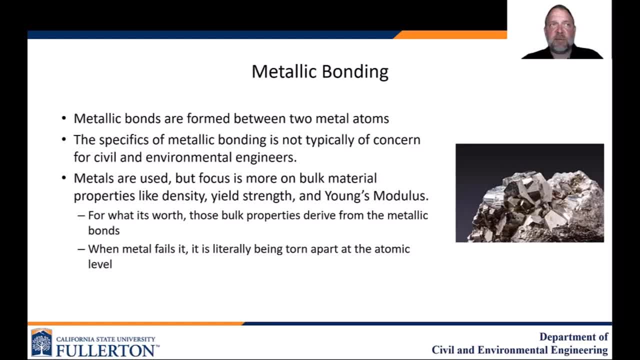 come from metallic bonds. So we can figure out how dense, we can measure how dense something is, we can measure how strong something is, and then that actually is derived from metallic bonds. When you destroy some steel, when you pull steel apart, it's actually being torn apart at the atomic level. 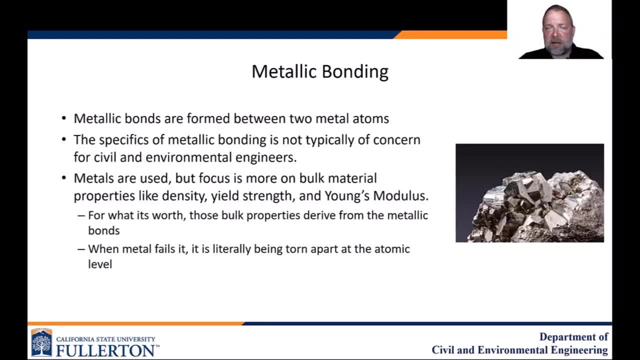 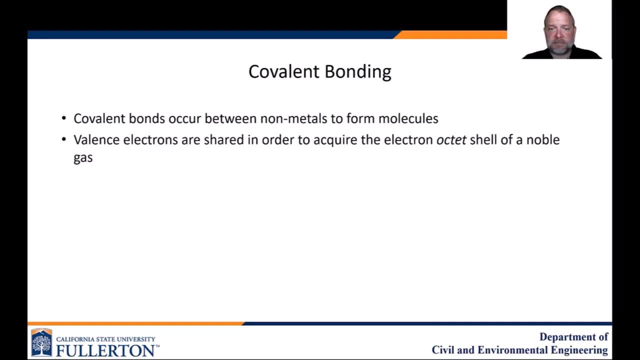 So it really is a metallic bond that's holding it together, but we only really care how strong it is. We can build buildings out of it. Covalent bonds occur between non-metals to form molecules, So you expect to see, like CO2,, for example, is a covalent bond between two non-metals, Valence electrons. 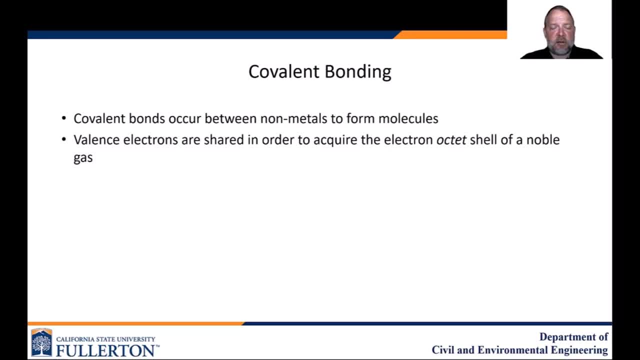 are shared in order to acquire the electron octet shell of a noble gas. With two exceptions, hydrogen and boron are other than eight, So most things like to have eight in their outer valence electrons. Hydrogen and boron are the two exceptions. We can use Lewis dot structures to. 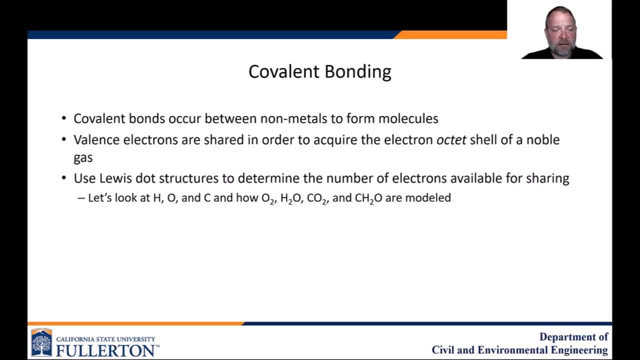 determine the number of electrons available for sharing. So let's look at hydrogen oxygen, carbon and boron and how they combine together to form diatomic oxygen that we breathe, water, CO2, and CH2O. So if you think about the Lewis dot structure for hydrogen, it's really simple. It's just a one. 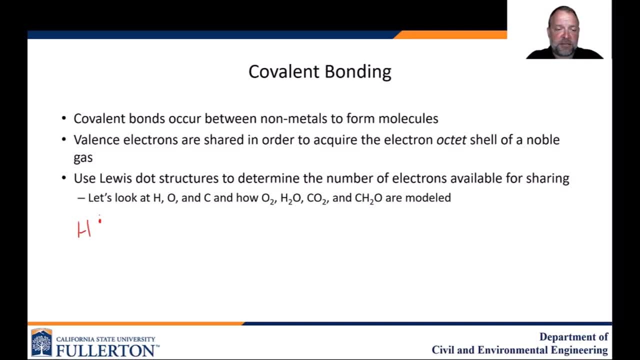 one dot. So that is the Lewis dot structure for hydrogen. For oxygen it's a little more complicated. Oxygen has six electrons in the outer shell: One, two, three, four, five, six. So it has two vacancies. basically It wants to have eight. 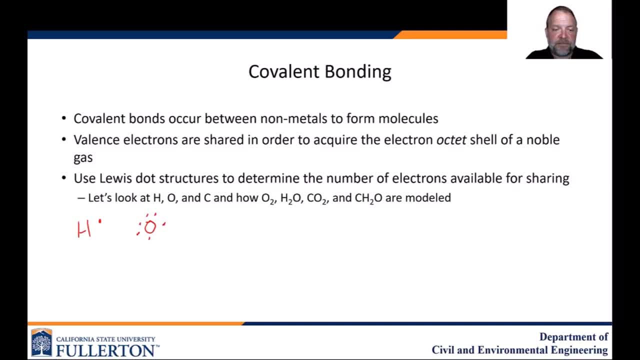 but it only has six. So there's two places for things to bond to oxygen. Carbon has four electrons in the outer shell And we can tell by the way. looking at the periodic table, we can see that everything in that group- carbon, silicon, germanium, tin- generally have 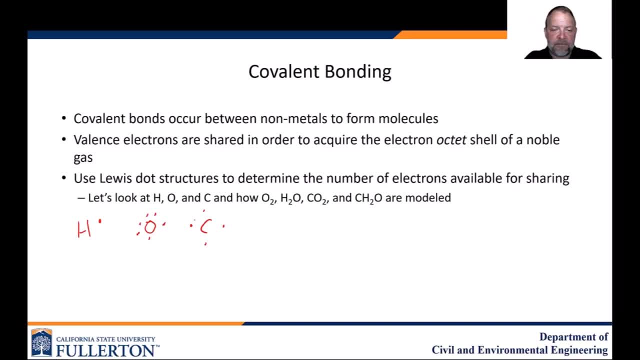 four electrons available in their outer shell because of the group that they're in. So we can look at these. So we have H, O and C, hydrogen oxygen and carbon And we can see how do they bond. So if we have, we want to make oxygen, O2.. Oxygen is actually a double bond, So it's got. 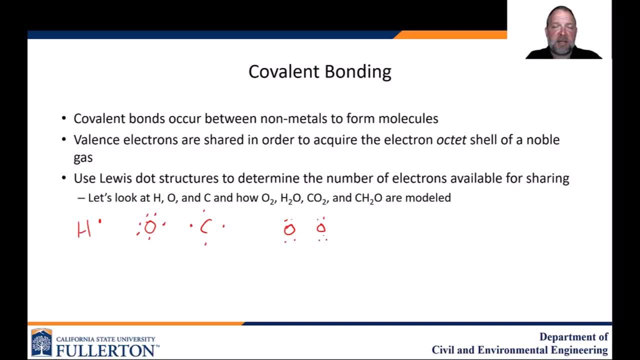 each one has the four electrons. that are happy. They're kind of just doing their own thing, But it has, it's missing two. And so it actually in a way you can kind of think about like one electron shares- sorry, one oxygen atom kind of like shares two electrons and the other one. 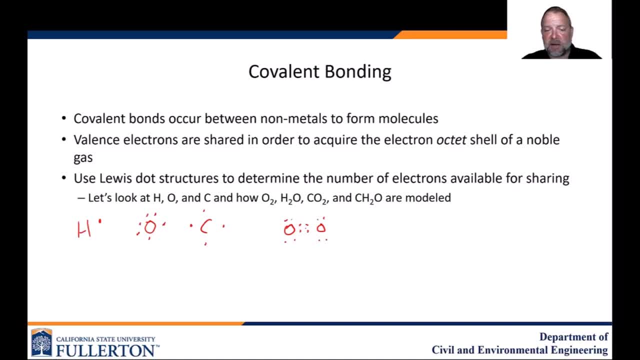 holds onto them, But because they're sharing, because now they're. if you look at their individual electron clouds, like if I look at just the cloud of oxygen, it's like oh, oh, oh, oh, oh electron clouds. Like, if I look at just the cloud of this one, it has eight electrons that I was 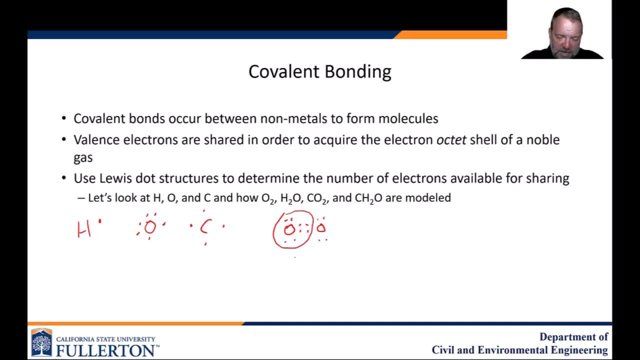 trying to get. And if you look at the oxygen- not the oxygen but the electron cloud of the other ones- I'll just erase this circle so you can see what I'm talking about- If you look at the electron cloud of the other oxygen, it also has eight that it's experiencing, So it feels it's. 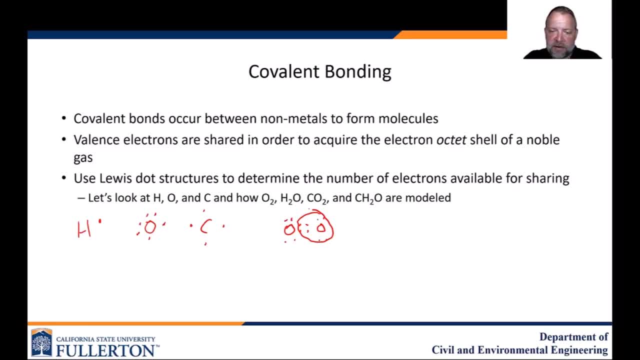 stable now because it has eight electrons. H2O is kind of similar. You start with oxygen. It's got four electrons that are not being shared, And then it happens to share two electrons with hydrogen. So now hydrogen is happy, It's got two electrons. That's what hydrogen likes to have. 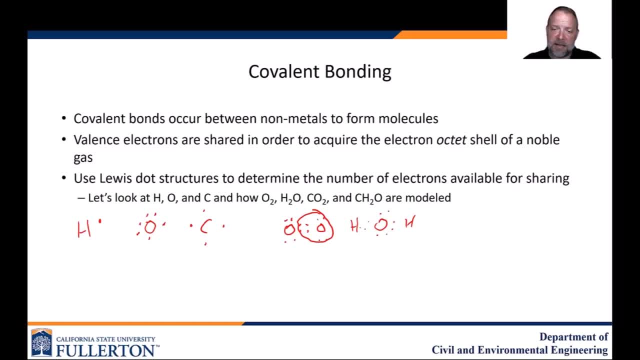 And then oxygen is happy because now it seems to itself that it has eight electrons- CO2, remember. carbon has four. It has four electrons, which means it's missing four. So it wants to hold onto four electrons from some other people. And oxygen is missing two. So oxygen and 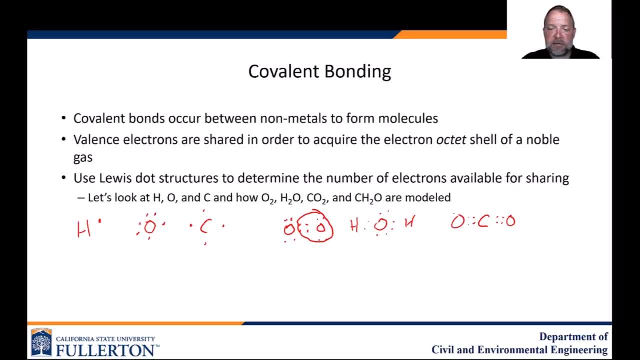 carbon actually form double bonds again in CO2.. And then for CH2O, again we start with our carbon. It's got something like this with the hydrogens and the oxygen: It still likes to hold two electrons from oxygen and two electrons, or one electron, from the hydrogen. And if you look at the 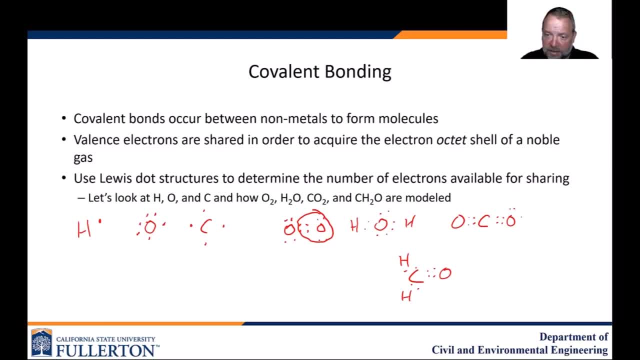 individual shells. well, you know, I forgot to draw in the the rest of oxygens. So if you look at the individual atoms, every one of them has the number of of uh electrons that likes to have. but you know what I drew: too many, Whoops. 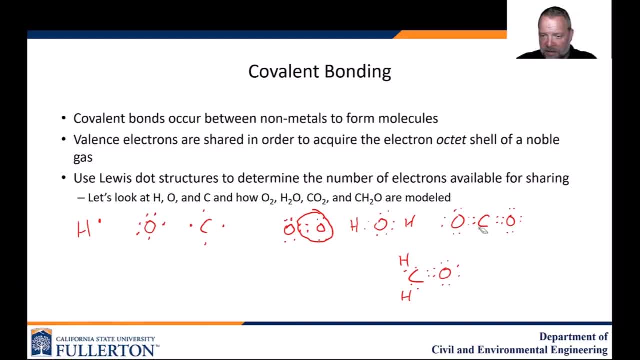 Let's go back, See, even even professors can make mistakes. So now everyone has the number of electrons they'd like to have. So you look at oxygen, it's got two, two, four, six, eight, two, four, six, eight. Carbon has one, two, three, four, five, six, seven. 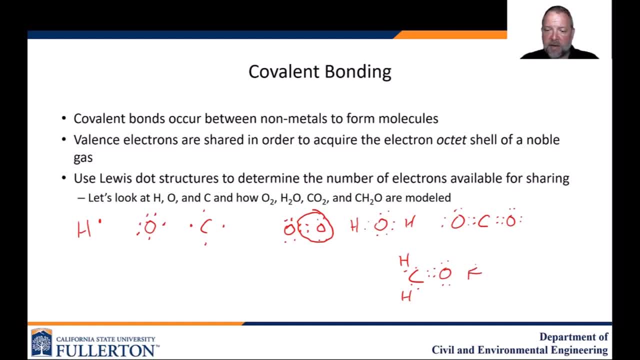 eight. Excellent over here on this one. Oxygen also has eight, carbon has eight. everyone's happy, And there will be one. the one. your practice problems will be to draw a Louis Depp structure. So keep that in mind, Just keep the slide in. 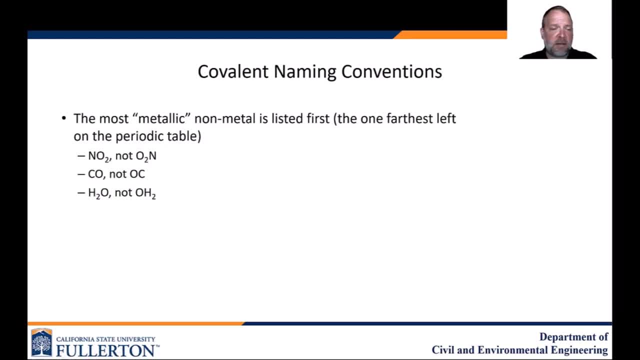 mind. I should say The way we name covalent bonds, covalently bonded material. I should say the most metallic non-metall exploit first. covalently bonded components: Delong-V sobriety bond B lot listed first. so one farthest left on the periodic table, like nitrogen, is farther left than oxygen. 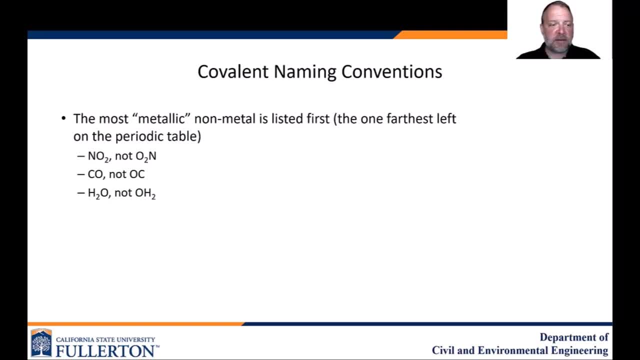 so it's no2, not o2n. carbon is farther left than oxygen, so it's carbon monoxide, not oc, oxygen carbide. and then hydrogen is farther left than oxygen, so it's h2o. we use prefixes to indicate the number of atoms, such as mono, di, ta, tri, tetra. you can read those if you want. 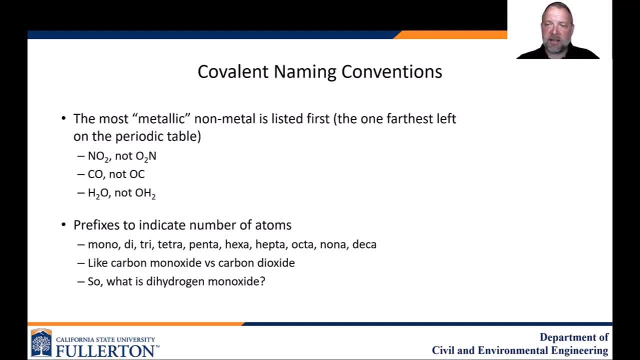 carbon monoxide versus carbon dioxide. that tells us that it's co versus co2. so co2 would be carbon monoxide. is this carbon dioxide? is that so that that di d i just implies there's two? so what is dihydrogen monoxide? well, it's h2o. 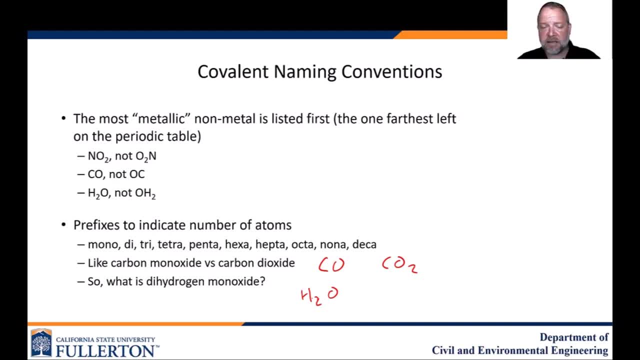 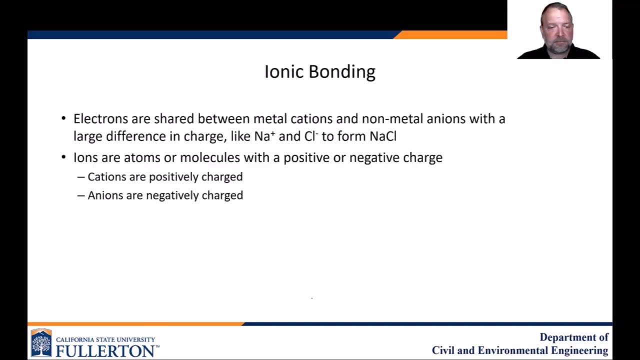 dihydrogen, two hydrogens, one oxygen monoxide, mono oxide, and then also that that i'd so ide gets added to the end of the second molecule. so carbon dioxide, it's not. it's not carbon dioxygen, it's carbon dioxide switching gears. we were talking about covalent bonding for a while there, but now ionic bonding. 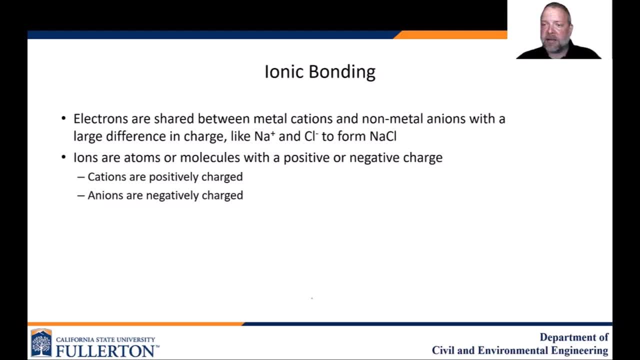 is when you have a bond between a metal cation and a non-metal anion. previously i mentioned that covalent bonds occur between two non-metals. ionic bonds occur between a metal and a non-metal with a large difference in charge, like in a large difference, like plus one. may not seem like that's. 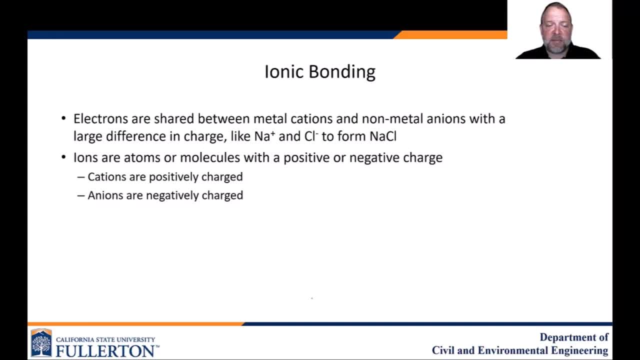 big of a difference, but it is so. sodium and chloride. sodium is a plus one charge, chloride has a minus one charge, so you get sodium chloride that forms, and that's that's an ionic bond. ions are atoms or molecules with a positive or negative charge, so anything that's charged could be called. 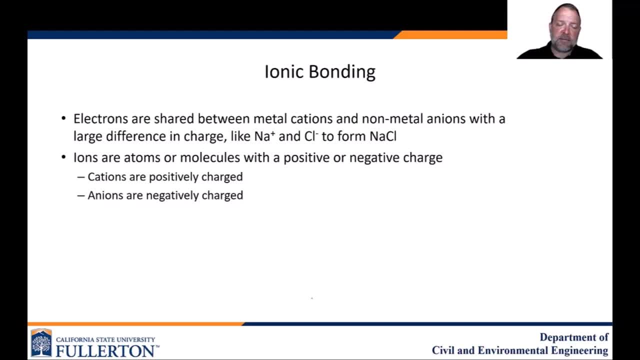 an ion, cations are positively charged, anions are negatively charged. i remember which ones which, by looking at this, so this a- t kind of looks like a plus sign, so positively charged, and an is in negative. So an anion is negatively charged, a cation, a T kind of looks like a plus sign. so that's how you can remember those two. 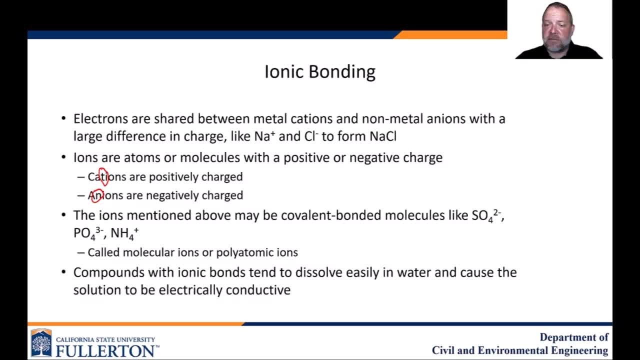 The ions above might actually be covalently bonded molecules. So something like sulfate SO4 here is covalently bonded. It's two nonmetals that are covalently bonded together, but because it has a minus 2 charge on it, it can actually bond with other things. 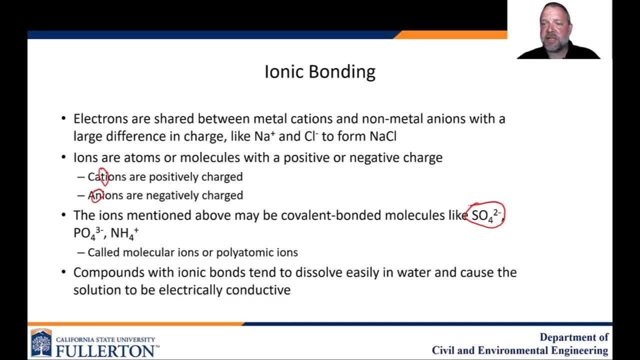 So you can get sodium sulfate, hydrogen sulfate. Hydrogen sulfate actually is sulfuric acid, So H2SO4, two hydrogens because you have a plus 1 charge on hydrogen, one sulfur because there's a minus 2 charge on sulfate. 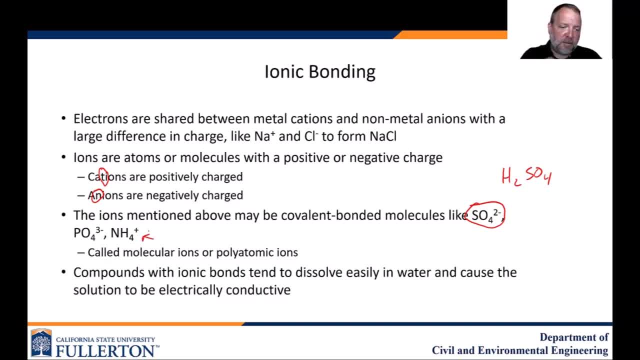 Same thing with phosphate. and then even there's a couple- only one- that I can think of off the top of my head. that's actually a cation. So ammonium is a cation because it has a plus 1 charge. So you can actually get ammonium sulfate probably in a 4, 2 SO4.. 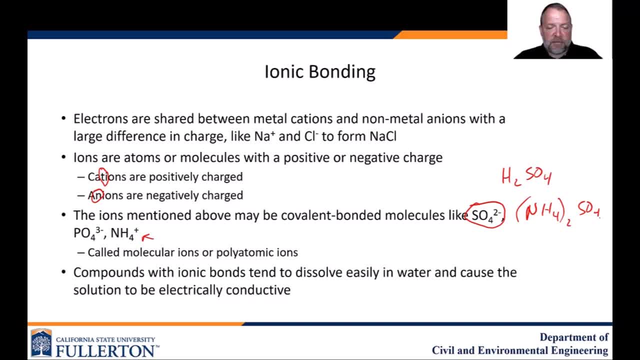 So you could, I think, have ammonium sulfate form. These are sometimes called molecular ions, I learned I always called them polyatomic ions, meaning that they are, they're like ions, they're, they're charged, but they're a molecule, not a, not an atom. 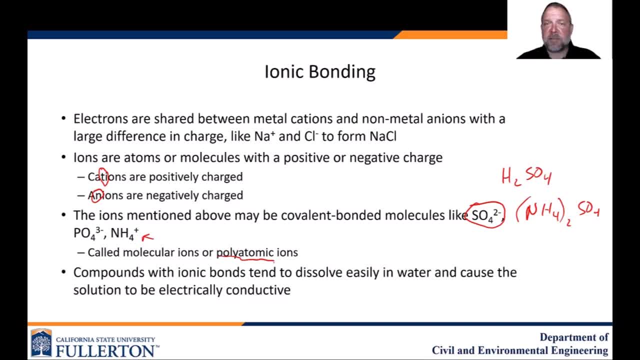 Compounds that have ionic bonds tend to dissolve easily in water and they also tend to make the water electrically conductive, And that has to do with the polarity of water. Water itself is polar. ionic compounds generally are kind of polar too. 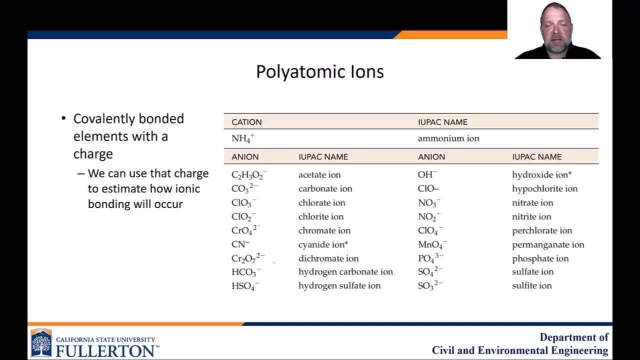 We'll talk about that in a second. Here's an example of a polar ion- Some of your polyatomic ions, or molecular ions, if you want to call it that. it's a covalently bonded element with a charge, So we can use that to estimate how ionic bonding will occur. 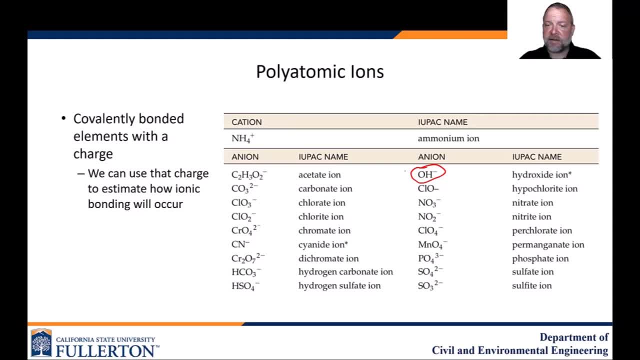 So, for example, if we have hydroxide over here, see, hydroxide has a minus 1 charge. So if you're combining hydroxide with sodium, it would be sodium hydroxide, because sodium is a plus 1 charge. hydroxide has a minus 1 charge. 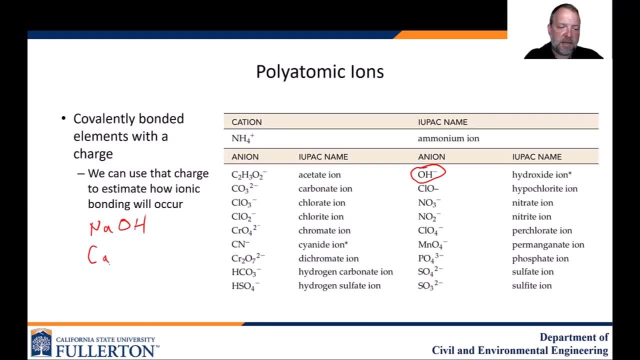 If it were calcium. on the other hand, calcium has a plus 2 charge, So it would be calcium hydroxide- is actually OH2, not CaOH. so it's CaOH2, calcium hydroxide, and I guess because it's not covalent- remember we talked about covalent ions, that you add, or, sorry, covalent compounds. you add, that I'd, or you add like the prefix, so you might think we would call this calcium dihydroxide, but generally speaking, it's not called that, it's just called calcium hydroxide. 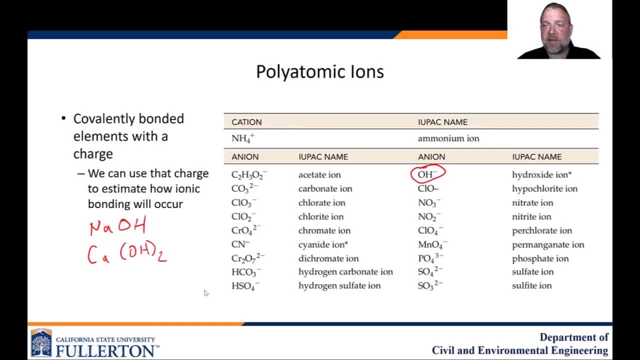 Oh, but there's a lot of. let me go back. there's a lot of different polyatomic ions. I did my PhD research on perchlorate, which I think is right here. yeah, so perchlorate is a oxidized form of chloride. 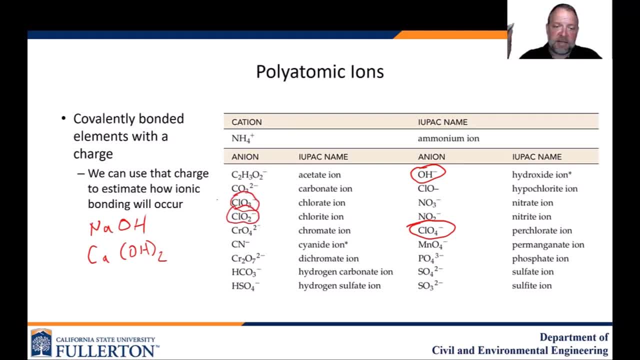 There's a lot of other ones that are oxidized forms of chloride too. So you have ClO3, ClO2, and ClO4, and it's weird because they all have a minus 1 charge, And then even there's one more, this one, ClO, also the minus charge, and you might recognize that term. 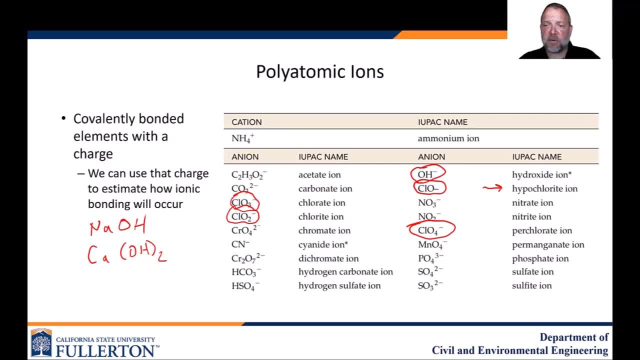 Hypochlorite is bleach, so calcium or sodium hypochlorite is what you buy when you buy bleach from the store. very, very reactive: it's a very active compound, so it breaks down the dyes in your clothes or kills germs. 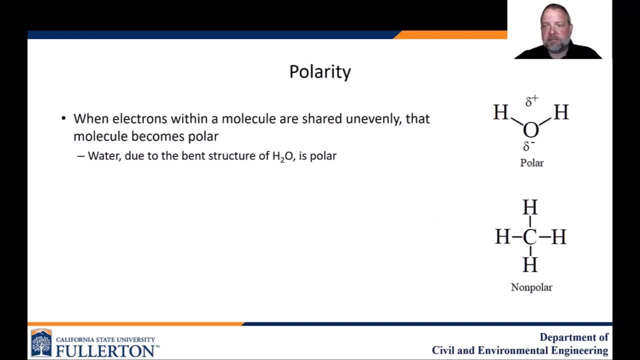 When electrons within a molecule are shared unevenly, that molecule becomes polar. polar, much like north and south pole of a magnet or north and south pole of the Earth. So you have hydrogen has a very, it's a positive charge, and oxygen is a negative charge. 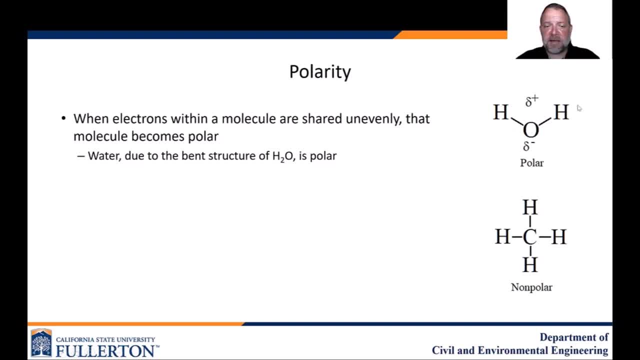 And when they come together, because it's not a symmetrical bond, it's a bent bond, a bent structure- because of that you get a slight differential positive charge, so a slight differential positive charge on the hydrogen side and a slight differential negative charge on the oxygen side. and so, because it's polar, it's able to dissolve things and kind of interact with things that are also polar. 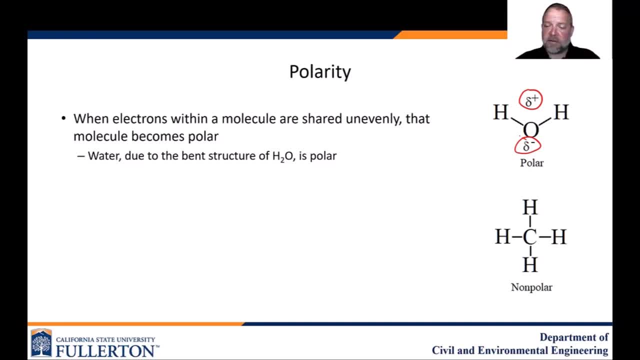 They like to have that slight charge difference. Something like methane, CH4, down here on the right is nonpolar because it's totally symmetrical. the way that hydrogen bonds to carbon in this case is a symmetrical bond. 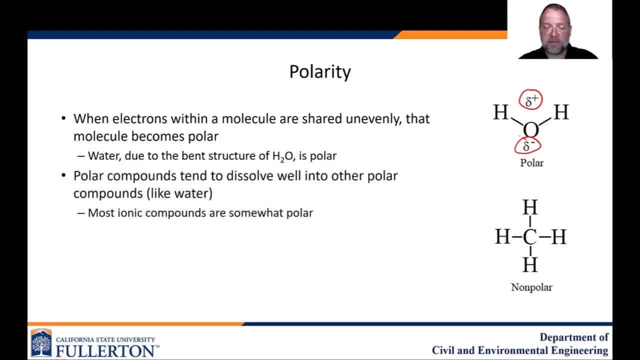 Polar compounds don't dissolve well. so most ionic compounds are somewhat polar, because they're a plus and a minus and they tend to share that unevenly. But then nonpolar compounds, so most covalent compounds are nonpolar. If you think about fats and greases, those are nonpolar compounds and they're also. they do not dissolve well. 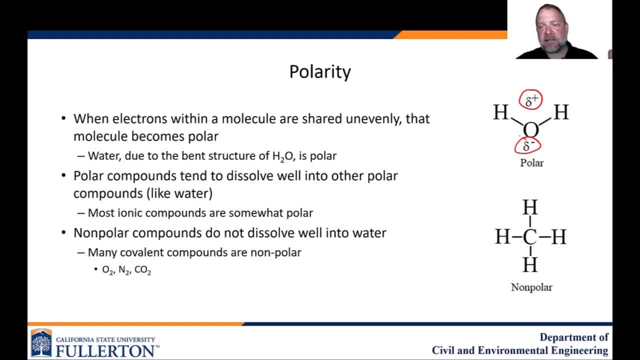 But if you take a fat and you cleave off the fatty acid and make it and put a positive charge there, it actually becomes a soap. It actually becomes so polar and because it's polar it's able to dissolve in water and so soap is made by taking fats and making them polar. 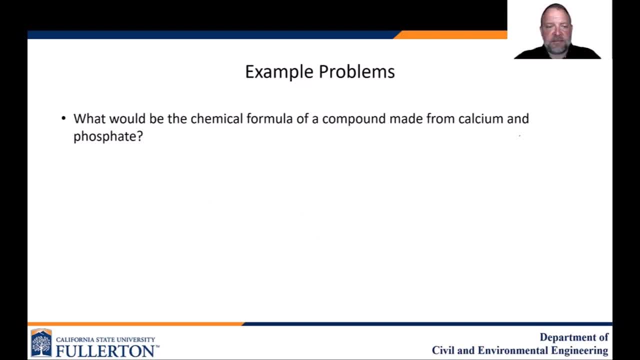 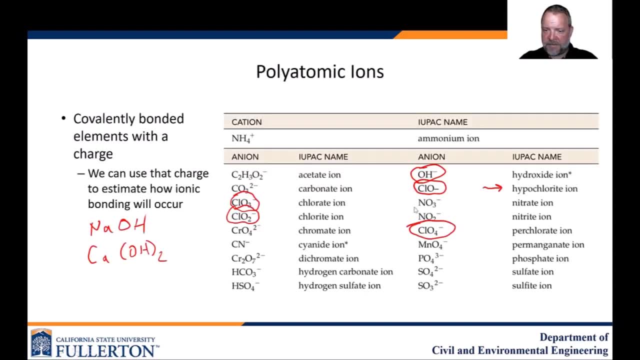 What would be the chemical formula of a compound made from calcium and phosphate. Okay, so we can go back. let me just scroll back, actually a couple slides and look what phosphate is. So phosphate, PO4, with a 3 minus charge. 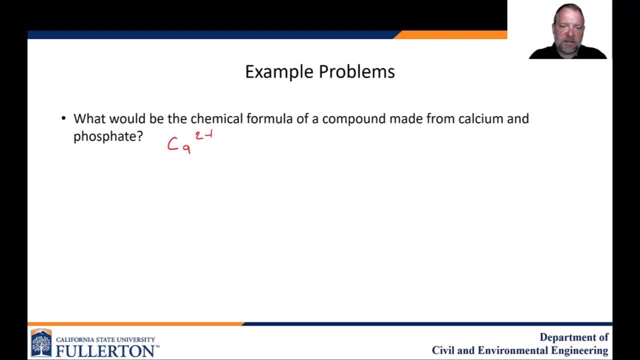 So calcium is a plus 2, we can tell that by looking at our periodic table. plus 2, it's in the second group. plus 2 charge. phosphate is a negatively charged, with a minus 3, that's supposed to be a 4, sorry. 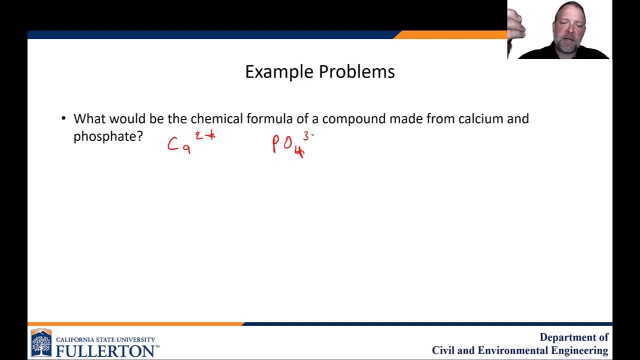 Never very good at writing on these screens Calcium phosphate, and so the way it would combine is you need 3 calciums for every 2 phosphates, so it's going to be a 3 to 2 ratio, And we just write that: like this, calcium 3.. 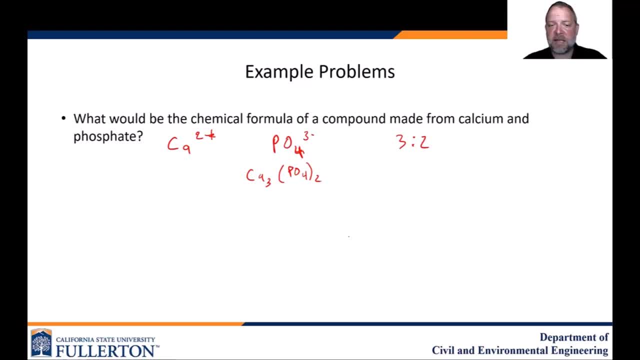 And if you think about that, now you have 6 positive charges and 6 negative charges and so it cancels out and they're able to bond together in that ratio. So the ratio is really important for this and the way you would write it. you could write the equation like this: 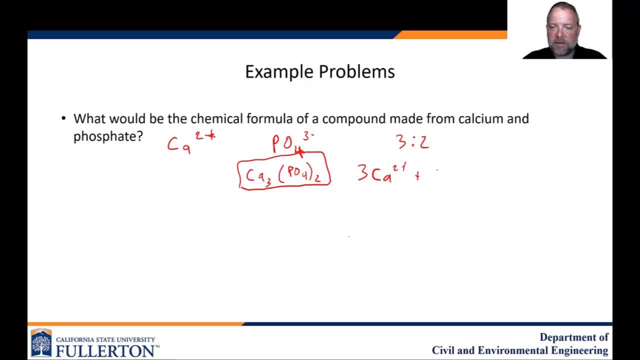 Calcium 2 plus So, 3 calciums plus 2 phosphate is in equilibrium with calcium phosphate. What is the name? and Lewis dot structure of a compound containing 1 carbon atom and 4 fluorine atoms. So fluoride is similar- or sorry, fluorine is similar to chlorine. it's in the same group. it also has 1 electron that it wants to share. 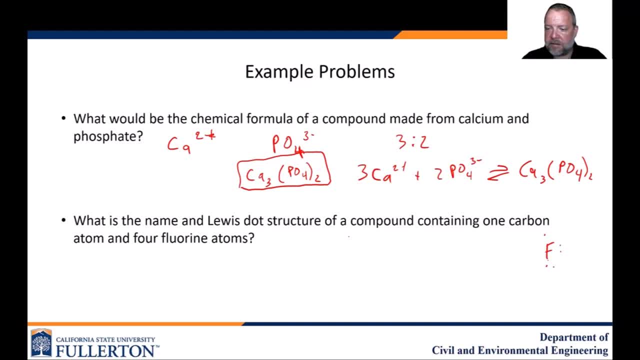 So fluoride has 7 electrons and it wants to have 8, so it needs to share one of those. it needs to borrow 1 electron from someone else. Carbon, if you recall, has 4 electrons. That means it has a vacancy. it's for 4 more, and so you get 4 chlorines- I'm sorry, 4 fluorines for every carbon. 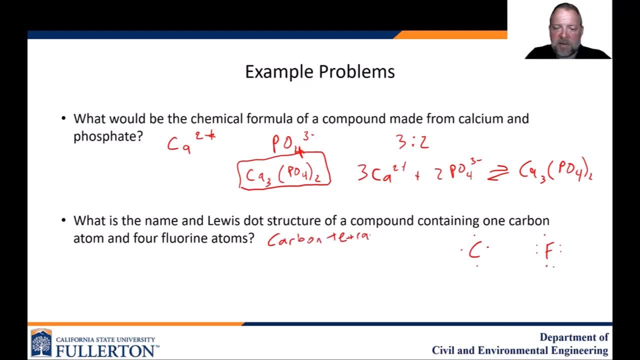 Now, if you remember, we talked about prefixes, because there's 4 fluorines, it would be a tetra. so carbon tetra fluoride- See I have. carbon tetra fluoride- See I have carbon tetra fluoride. 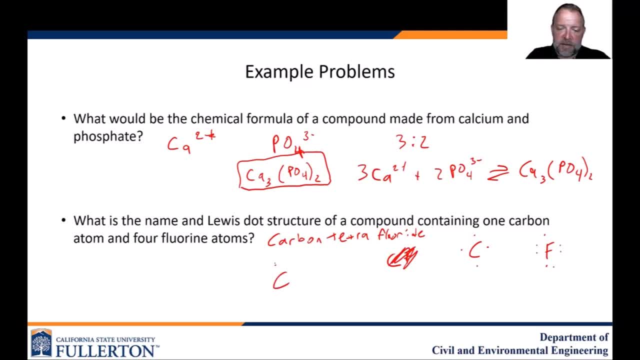 See, I have carbon, tetra fluoride. I should've known about that Carbon. as we said before, it has 4 electrons, Fluorine has 7, and 1,, 2,, 3,, 4,, 5,, 6,, 7.. 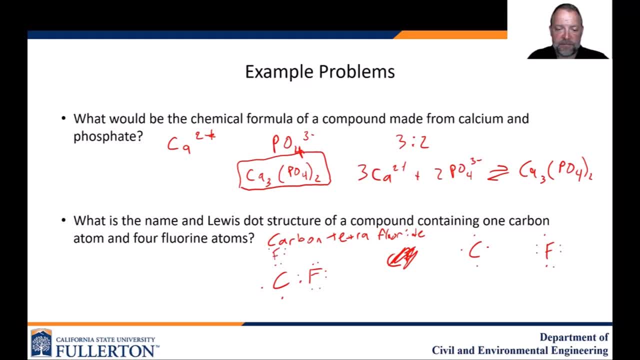 So fluorine will form something like this: Carbon tetra fluoride will look something like this: Now, all the fluorines, all the fluorines, have 8 electrons, that's 7. electrons that are being shared. the carbon has eight electrons being shared, and so it's a happy. 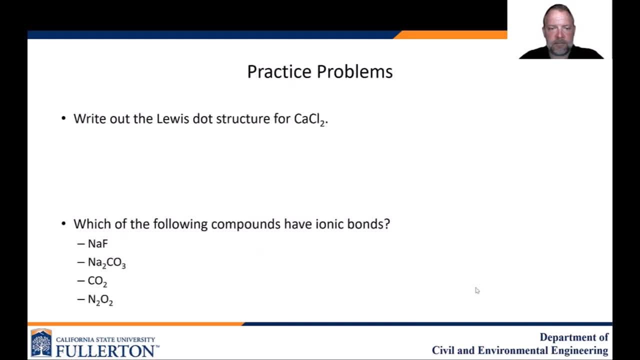 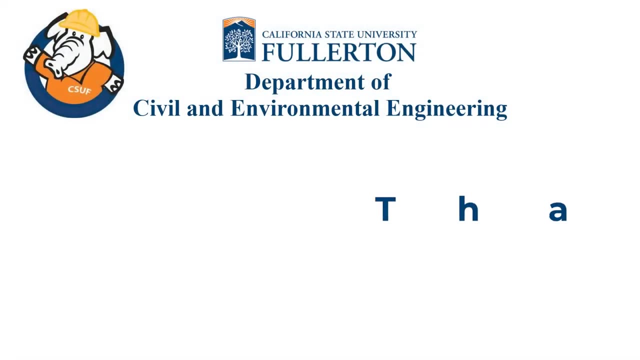 camper and last but not least, are some practice problems for you to uh work on your own all right. i hope that was useful for you and i know you'll be using stuff like this in your future classes. so thanks for your attention.